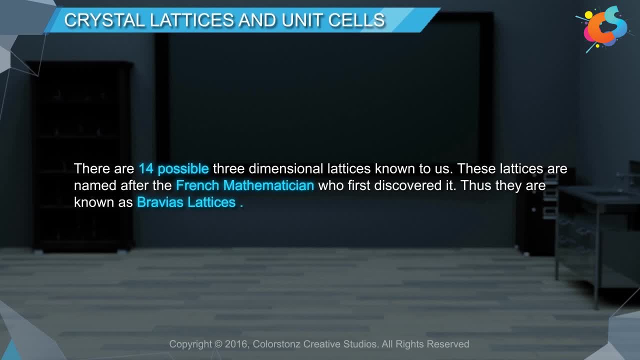 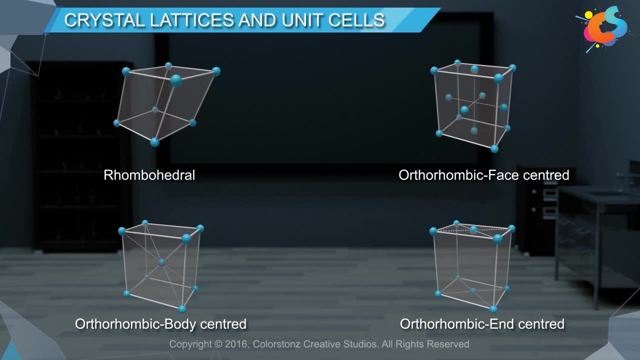 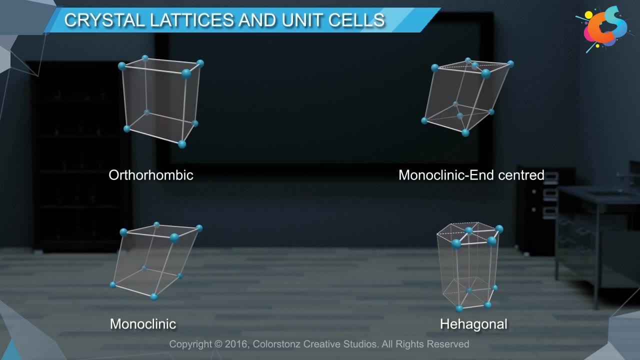 who first discovered it. Thus they are known as Bravias lattices. In addition to simple lattices for other systems, it is observed that there are 14 different types of space lattices. These are known as 14 Bravias lattices. 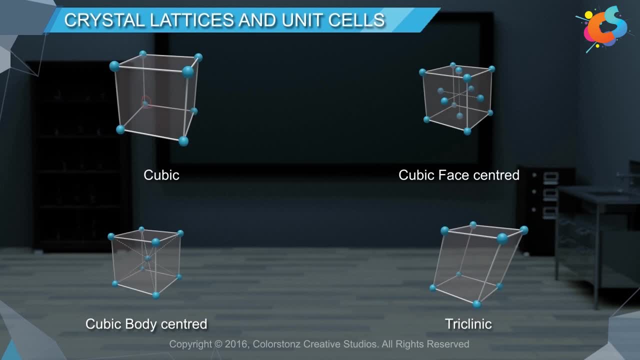 These lattices are known as Bravias lattices. These lattices are known as Bravias lattices. These lattices were given name after a French mathematician who first described them. Now we know what is a crystal lattice. 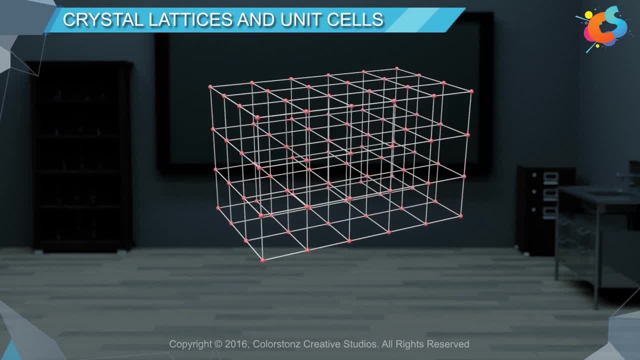 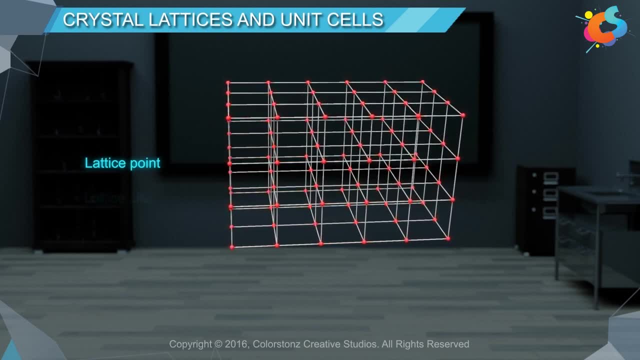 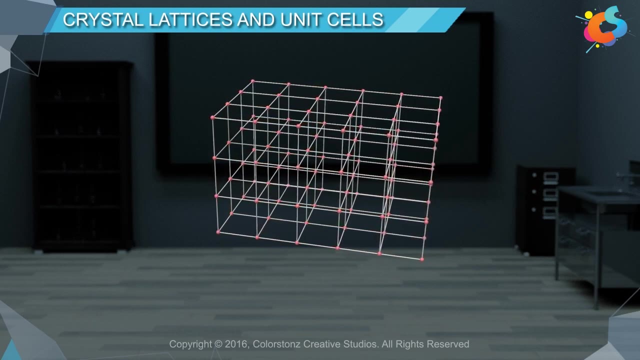 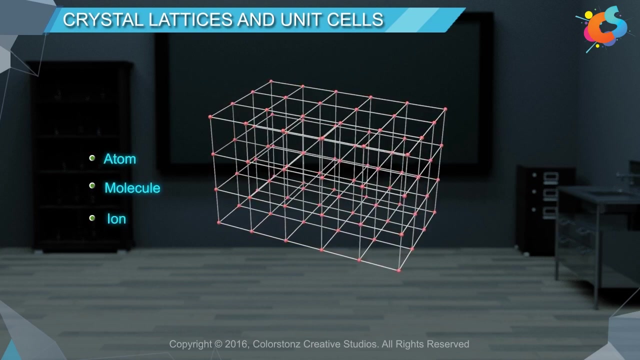 Let us study some of its characteristics. Each point in a crystal lattice is called lattice point or lattice site. Each point in a crystal lattice represents one constituent particle, which may be an atom, a molecule or an ion. Lattices points are joined together by straight lines. 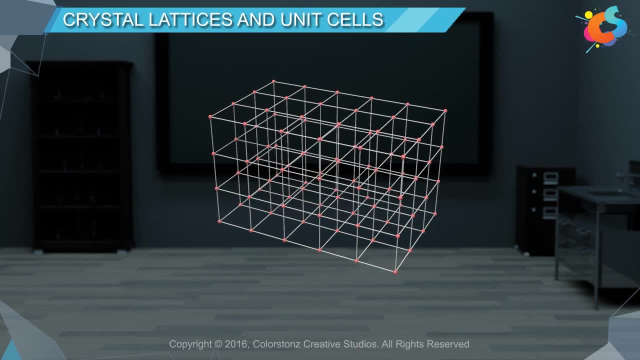 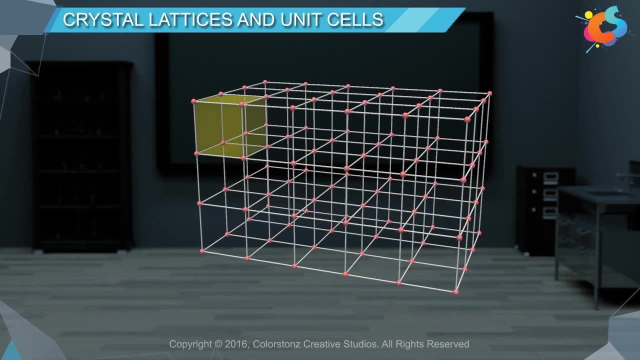 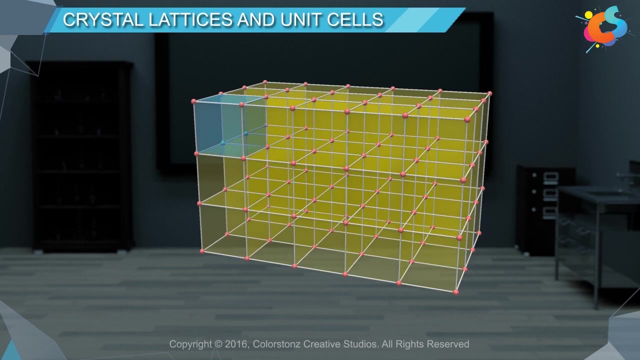 to bring out the geometry of a crystal lattice. Now, if we observe this crystal lattice, we can notice that there is a small group of lattice points that repeats itself again and again to form an entire crystal lattice. This small group of lattice points is known as unit cell. 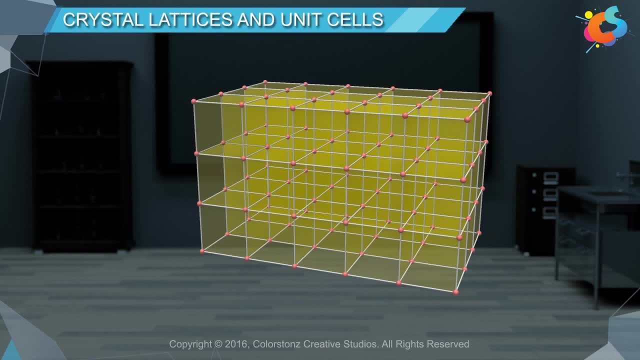 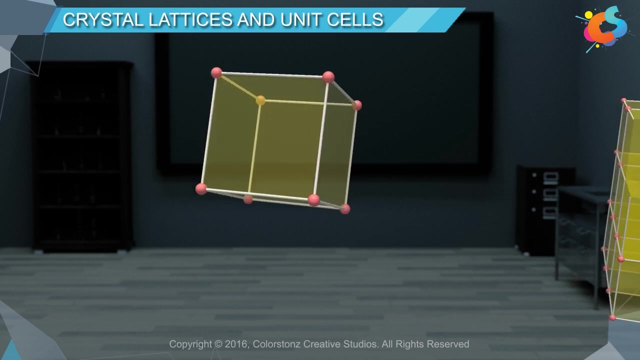 Thus, unit cell is the smallest portion of a crystal lattice. When repeated in different directions, generates the entire lattice. A unit cell is represented by three edges: A, B and C. Represented by three edges: A, B and C. Represented by three edges: A, B and C. 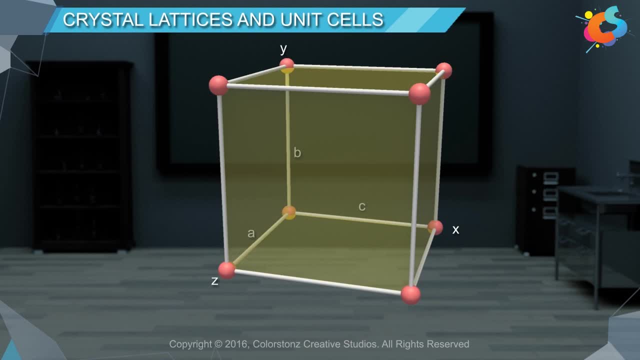 Represented along X, Y and Z axis of a three-dimensional entity And these edges may or may not be mutually perpendicular to each other. When these edges join, they form certain angles. They are represented as alpha, beta and gamma. The angle between edges B and C is alpha. 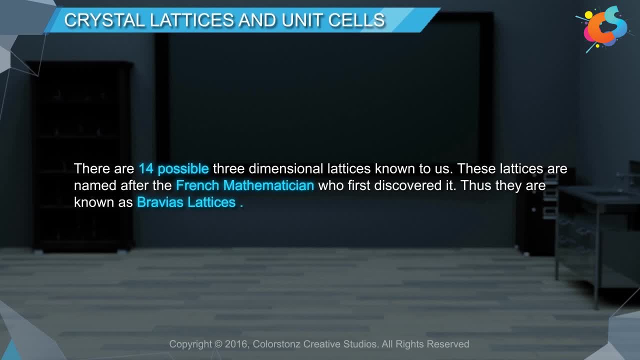 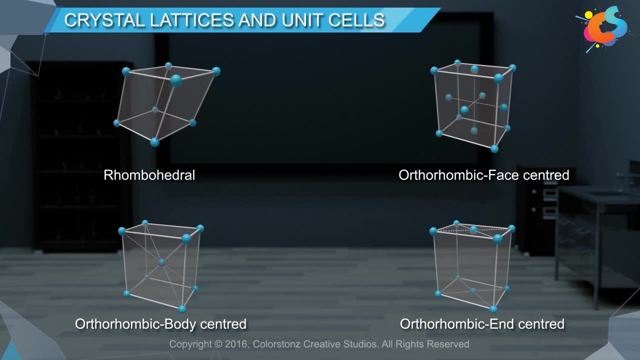 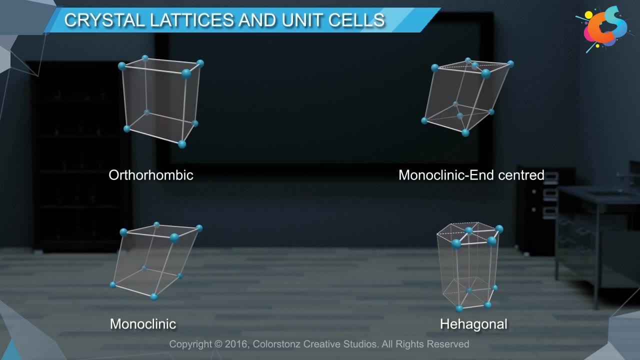 who first discovered it. Thus they are known as Bravias lattices. In addition to simple lattices for other systems, it is observed that there are 14 different types of space lattices. These are known as 14 Bravias lattices. 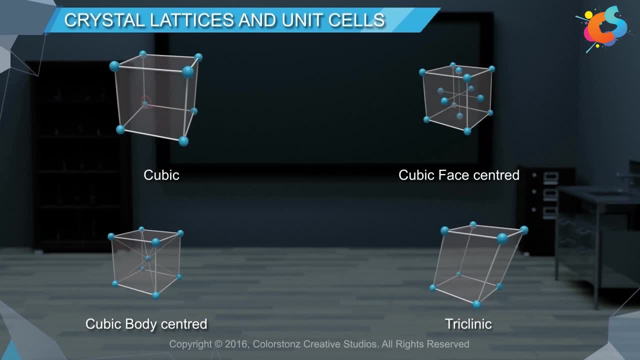 These lattices are known as Bravias lattices. These lattices are known as Bravias lattices. These lattices were given name after a French mathematician who first described them. Now we know what is a crystal lattice. 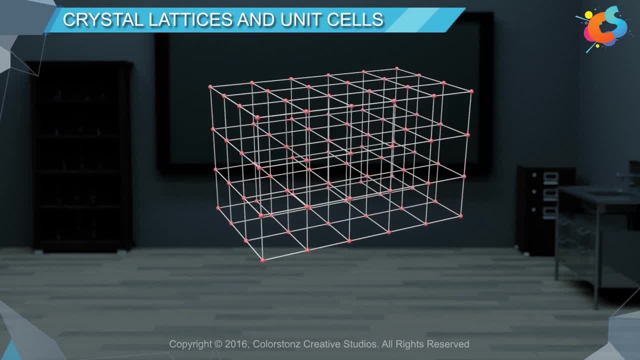 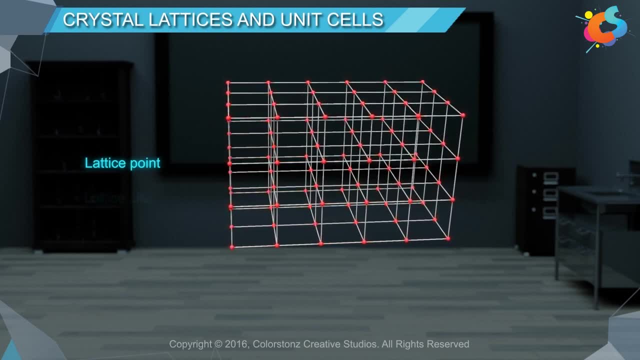 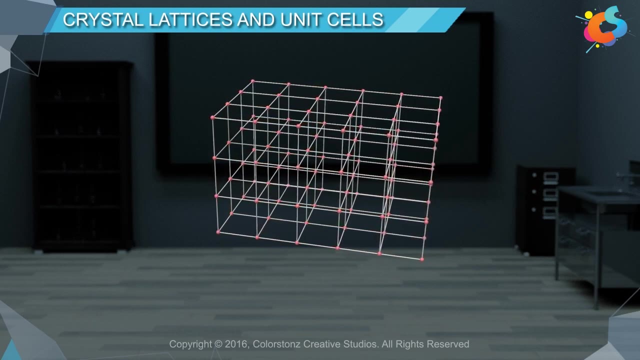 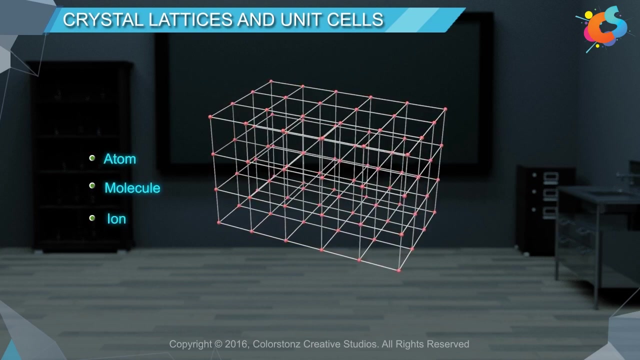 Let us study some of its characteristics. Each point in a crystal lattice is called lattice point or lattice site. Each point in a crystal lattice represents one constituent particle, which may be an atom, a molecule or an ion. Lattices points are joined together by straight lines. 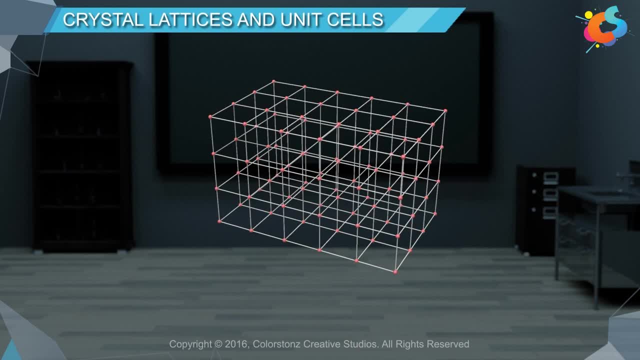 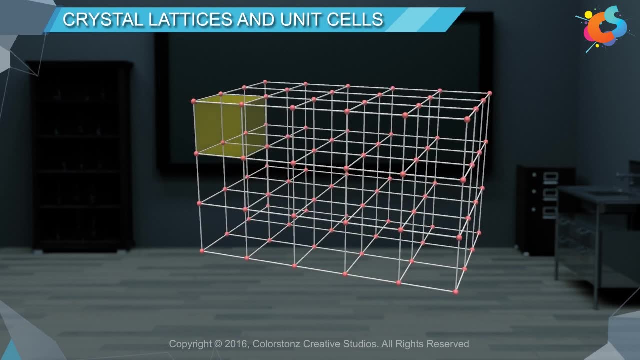 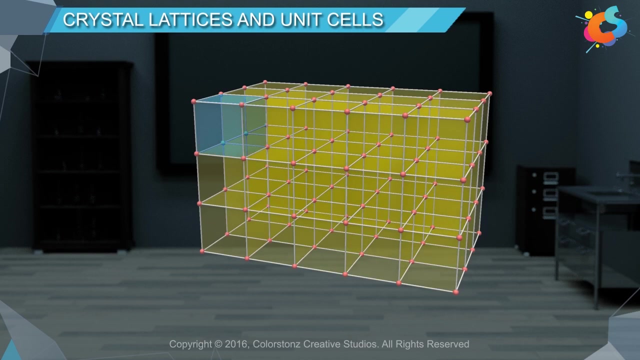 to bring out the geometry of a crystal lattice. Now, if we observe this crystal lattice, we can notice that there is a small group of lattice points that repeats itself again and again to form an entire crystal lattice. This small group of lattice points is known as unit cell. 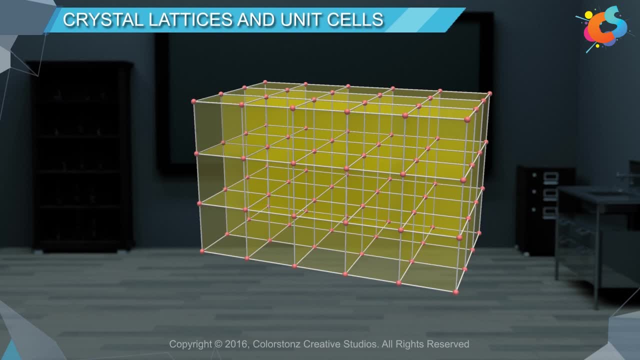 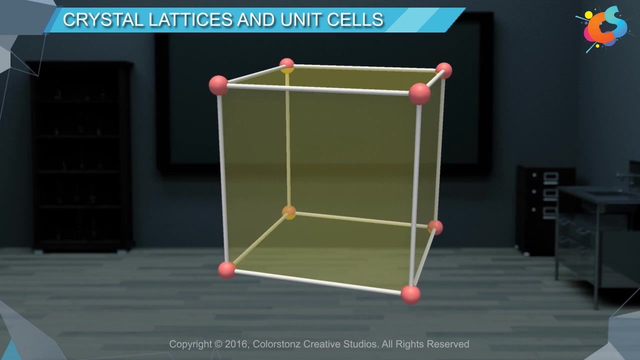 Thus, unit cell is the smallest portion of a crystal lattice. When repeated in different directions, generates the entire lattice. A unit cell is represented by three edges: A, B and C. A unit cell is represented by three edges: A, B and C. 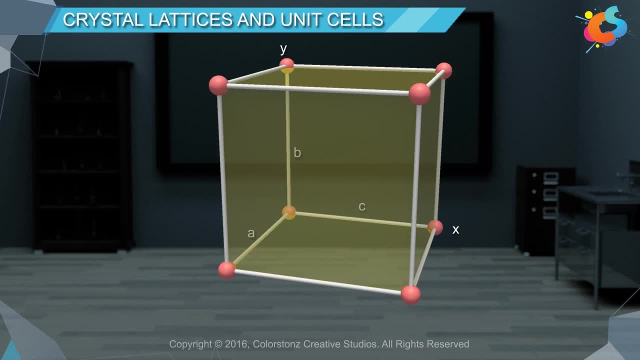 A unit cell is represented by three edges: A, B and C. Their heights are represented along along x, y and z axis of a three dimensional entity, and these edges may or may not be mutually perpendicular to each other. When these edges join, they form certain angles.